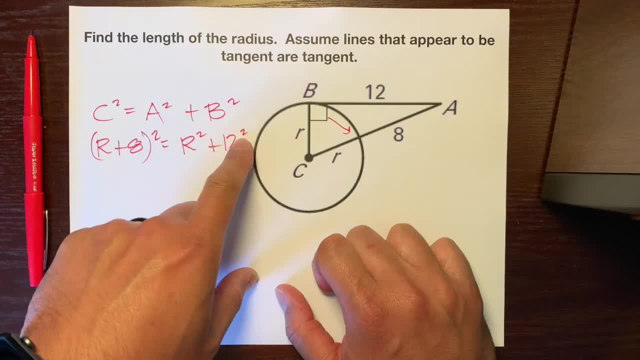 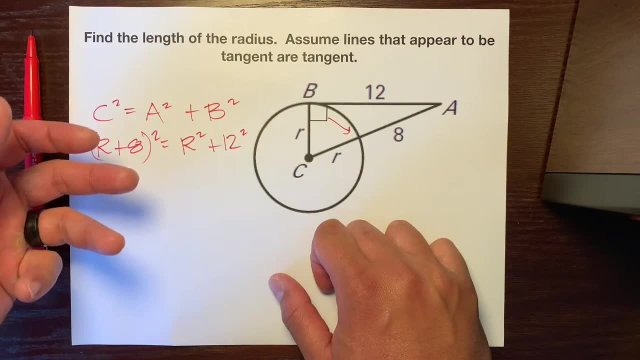 may do this. you may see, there's a square here, there's a square here, there's a square here. so we can just square root both sides. however, that breaks some rules. that breaks some algebra rules, because there's a plus sign right here. we can't square root both sides to get rid of all. 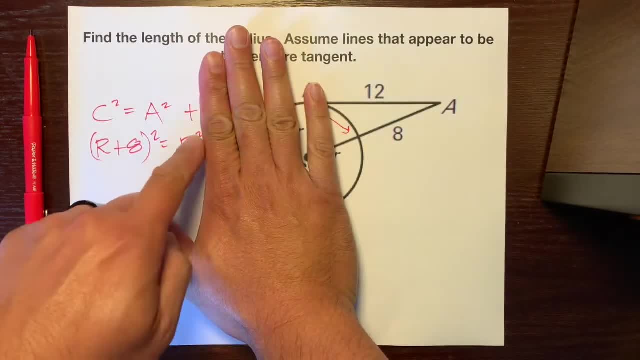 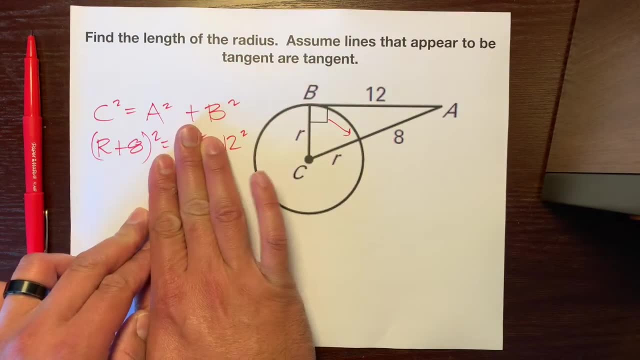 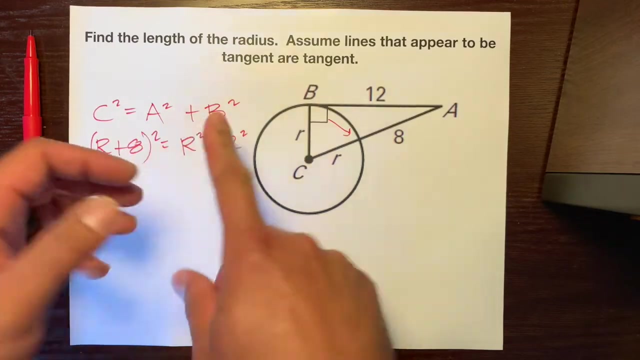 these squares right here. if it was just this, if it was just r squared and this, then that's fine, we could do that. or if it was just this and this, uh, we could do that. or if there wasn't a plus sign, if it was uh, r squared times 12 squared, then we could square root both sides. but the big thing, 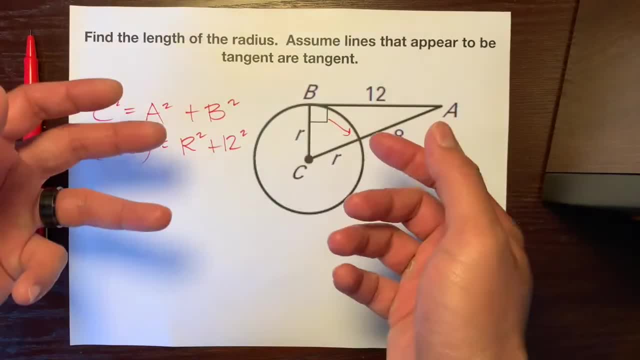 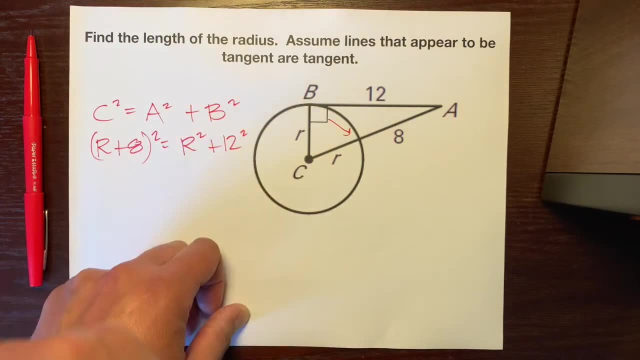 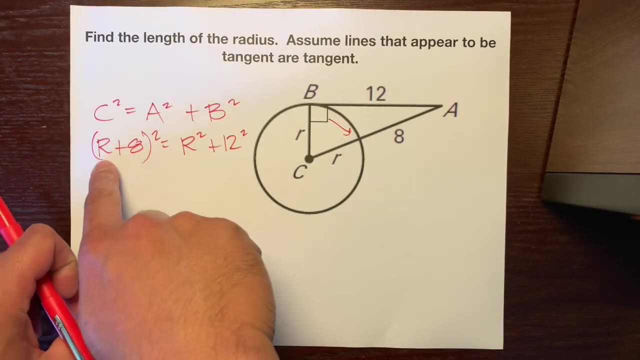 keeps us from being able to make this an easier problem. like you want it to be, like the world wants it to be, is this plus sign. so this plus sign says nope. you cannot square root both sides. so what we have to do is this: we have actually have to do some algebra. we have to work. 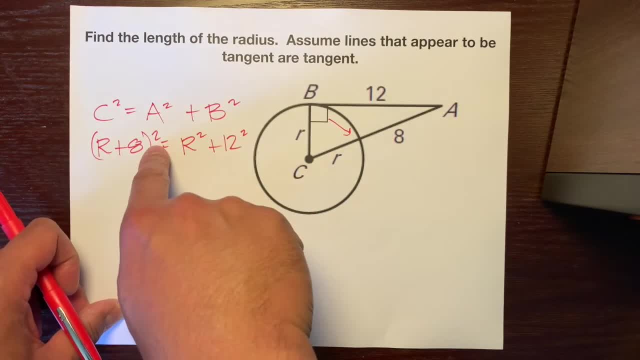 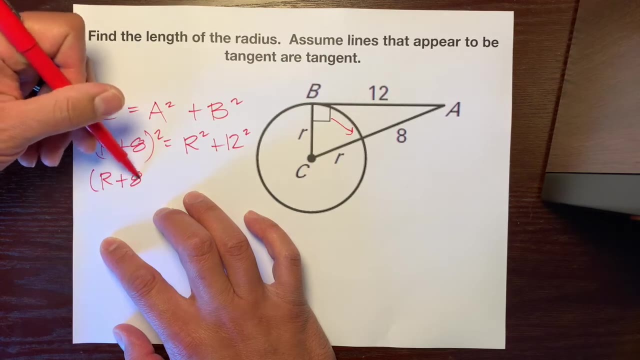 this out and again. uh well, not again, but for the first time. you cannot distribute this square into here and into here, because this plus sign, so these pluses make things a little complicated. so what we have to do is write r plus 8 twice, so r plus 8, times r plus 8. okay, so remember a square. 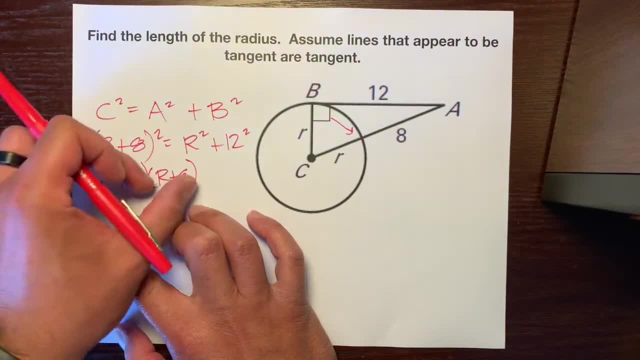 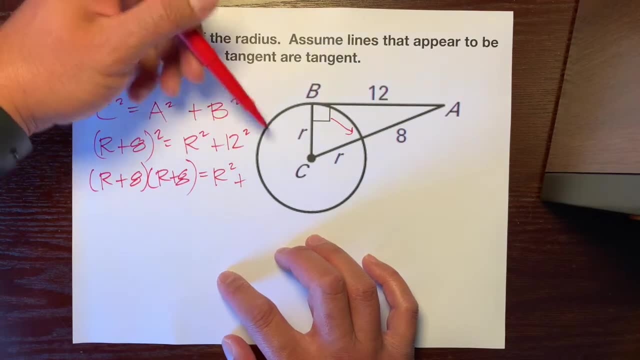 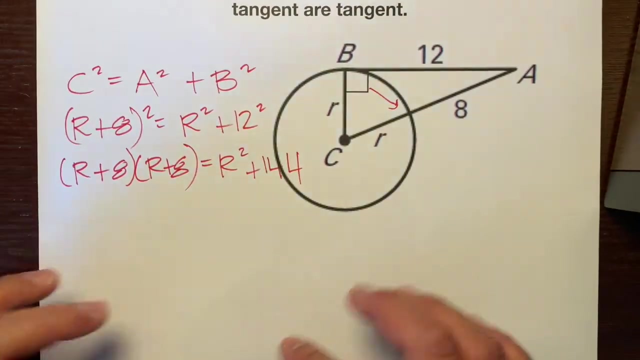 just means there's two. this is multiplying it by itself, so we just expanded it and we're going to r squared plus now, 12 squared is not 24, it's 12 times 12, which is 144. uh, and then what we're going to do is we're going to 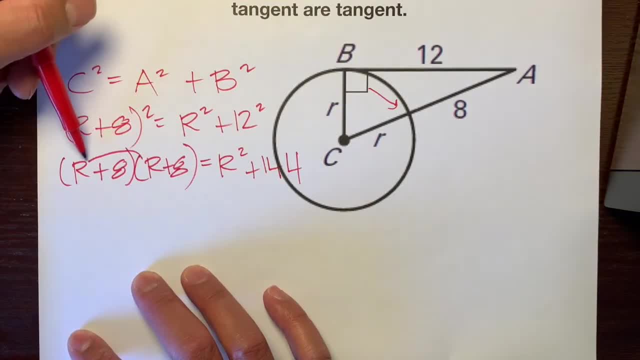 distribute twice, or foil, whatever you want to call it. so take this r and distribute it there, and we're going to take this 8 and distribute here and here. so let's distribute this r first. r times r is r. squared r times 8 is 8 r now. then we're going to distribute this 8 to here and here. 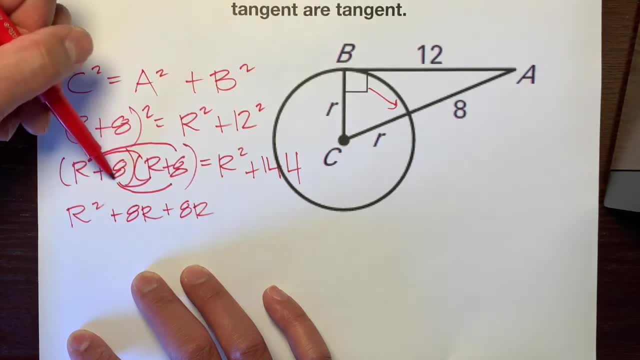 8 times r is 8r and 8 times 8 is 64. so this, this turns into this, which turns into this. the whole reason again, why we can't just square root both sides is because of the plus sign. if you did, you get a totally different answer, and that totally. 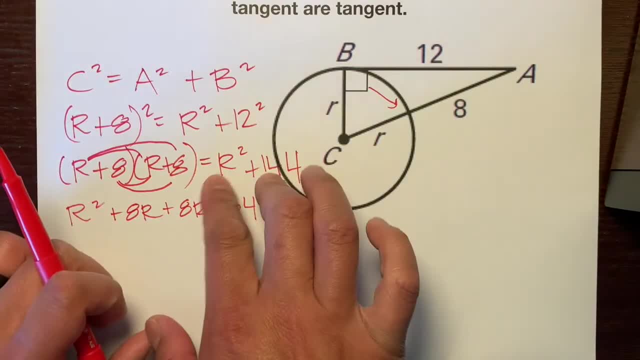 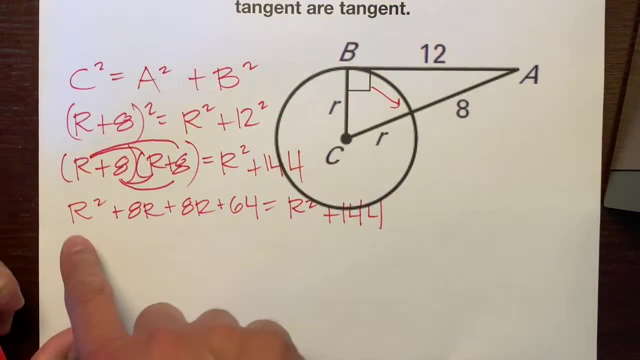 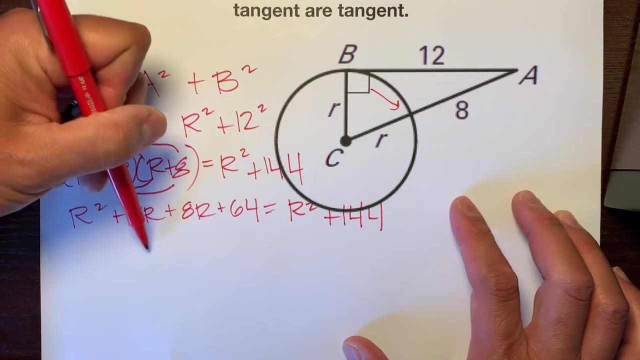 different answer would be totally wrong. so don't be totally wrong. next thing: bring down this r squared plus 144.. uh, now let's look at this side of the equation. let's see if you can combine any like terms. yeah, we can combine this: 8r plus 8r, which is 16 r. 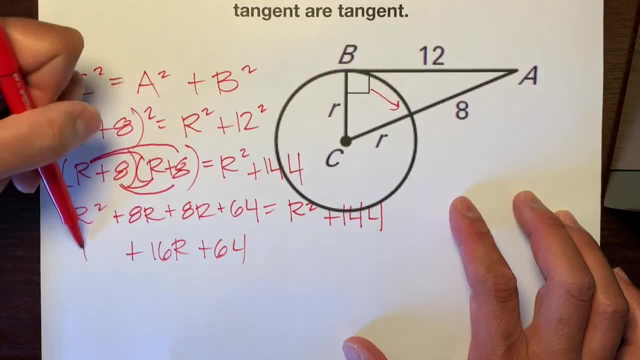 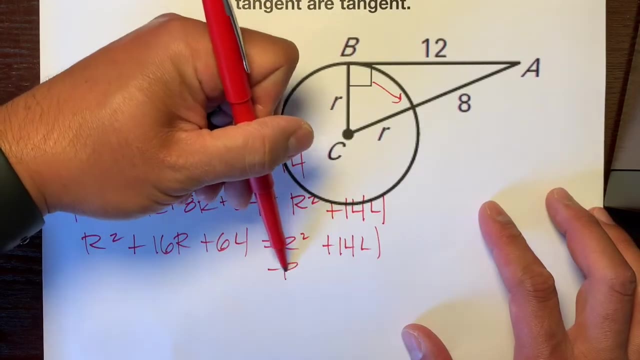 plus 64.. now we have this: r squared is equal to r squared plus 144.. and uh, let's get all the r's on one side. let's get this r squared. uh, let's get rid of it. so let's subtract this r squared from here. 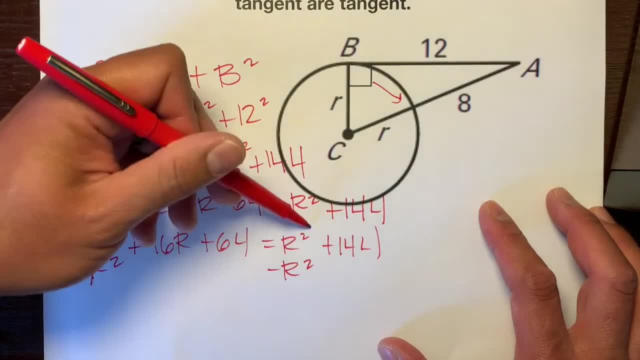 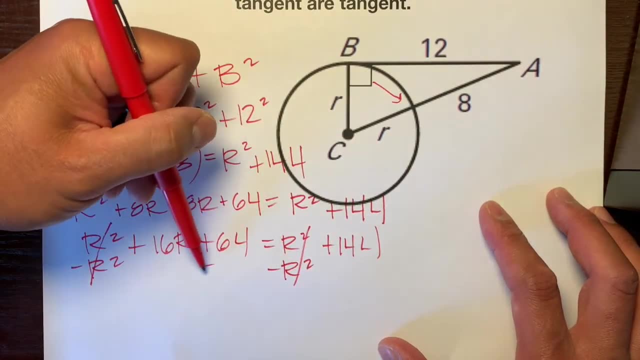 and to here it's like term and these actually cancel out. so it makes things a little easier and let's take the 64 and bring it to the other side. we have r's on one side and all the numbers without variables on the other side, and let's 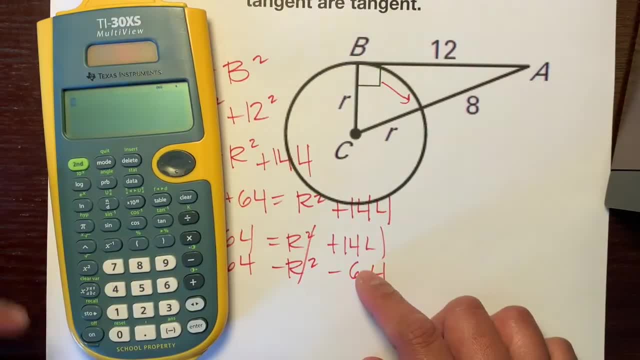 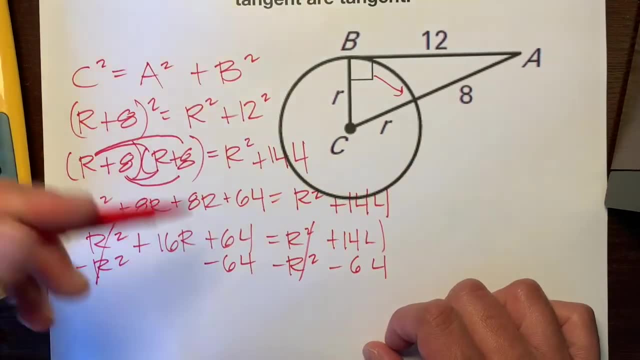 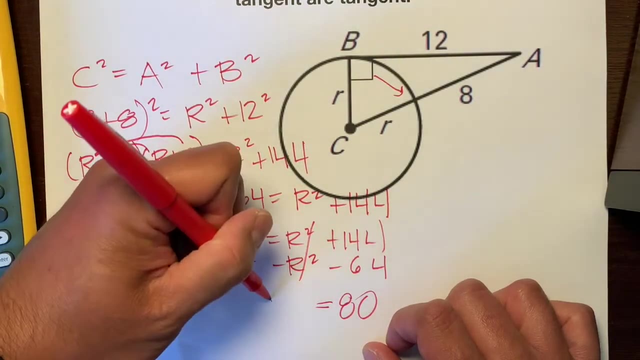 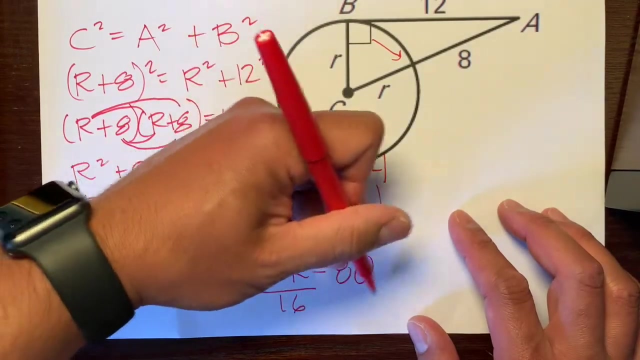 take our trusty calculator. hopefully we trust it: 144 minus 64 is 80, so we have so these. cancel out, this turns into 80 and this 16r we'll bring it over here, we'll bring it a little closer. and the last step: let's divide the 16 on both sides, and 80 divided by 16, i think it's five. 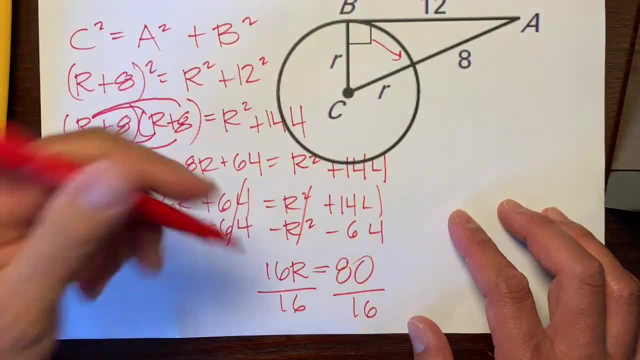 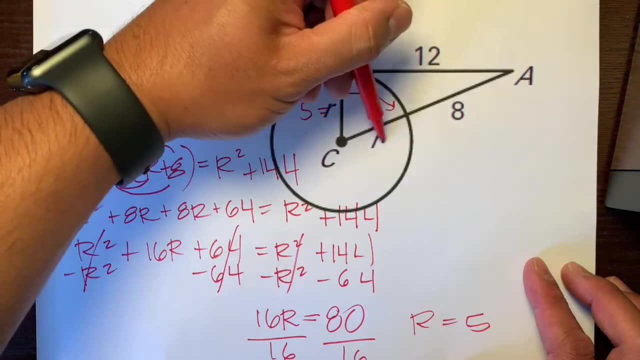 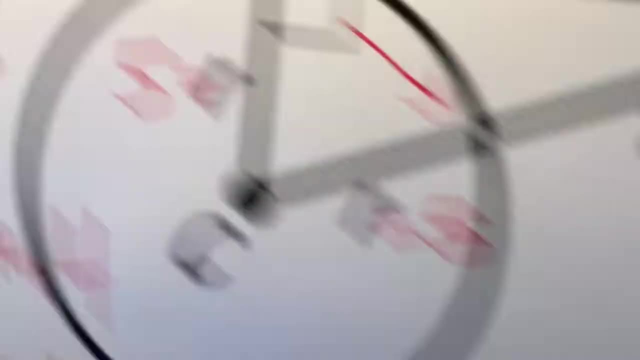 and yep, i beat the calculator. so r is equal to five. so the radius equals five. this radius equals five because all the radii are the same in the same circle. so here's your final answer: r equals five, there r equals five, there, five units. there's no inches. 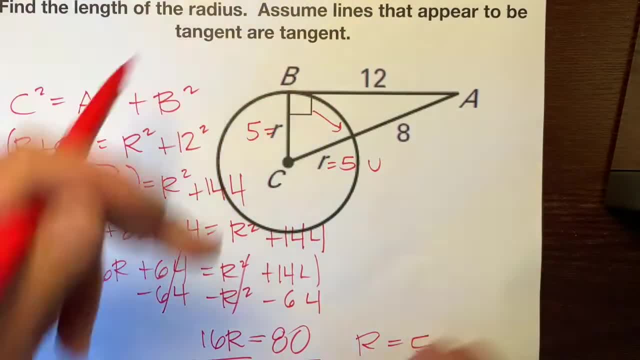 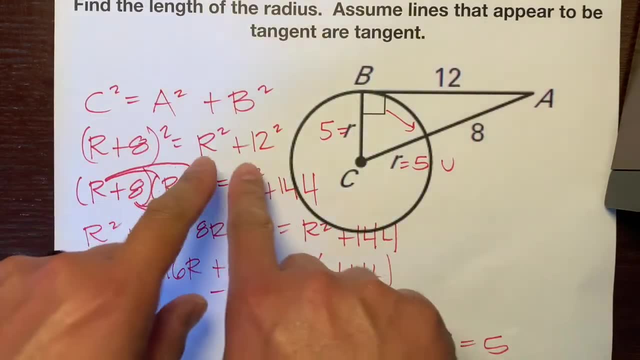 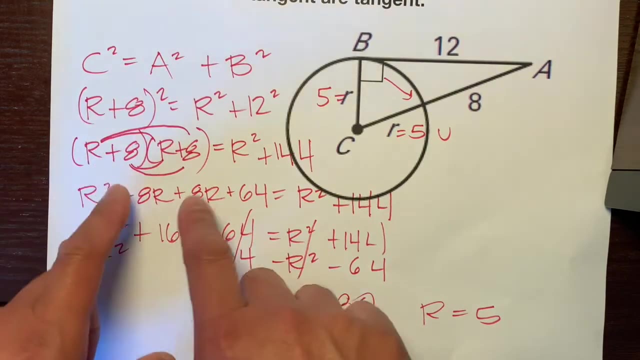 don't feed, so it's just five units and there's your final answer. so again, uh, don't, you cannot square root both sides because of this plus sign. um, so, and don't distribute this to here and here, because of the plus sign. you have to do some real algebra. so you get the correct answer and you. 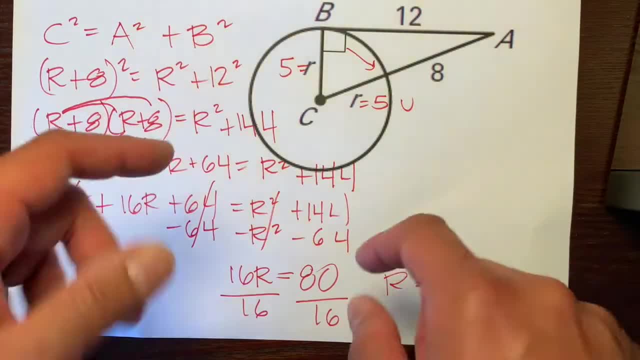 don't get a totally different answer, which is the totally wrong answer, get the totally right answer, which is five. all right, hope this helps. have a great day. bye.